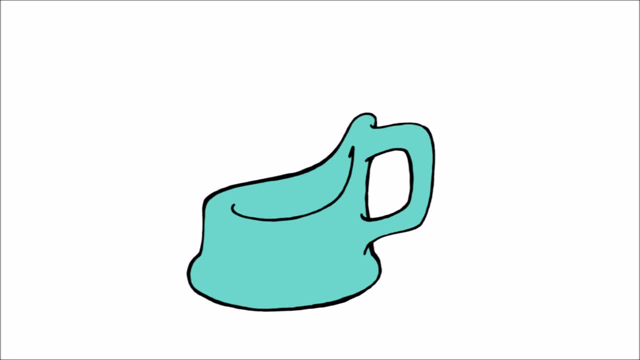 squishy rubber. then, when you're tired of drinking coffee from it, you can squish the cup part down until it collapses into itself, leaving only the handle which, as far as you're concerned, is indistinguishable from a delicious donut. Now you might be thinking: 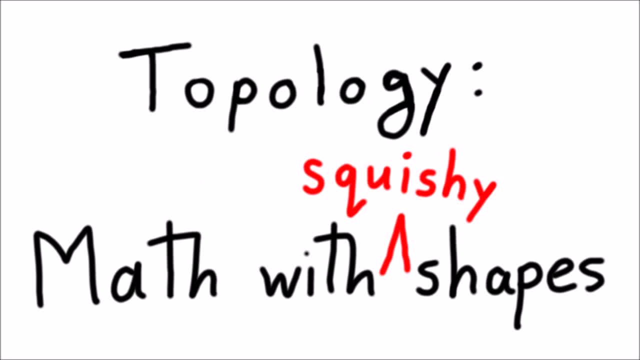 hey, but how is this math? If we're so relaxed in our definition of shape that we can't distinguish between a donut and a coffee cup, then how can we ever say anything meaningful or rigorous about the shapes we're studying? And that is an excellent point. One thing to note is that a topologist can: 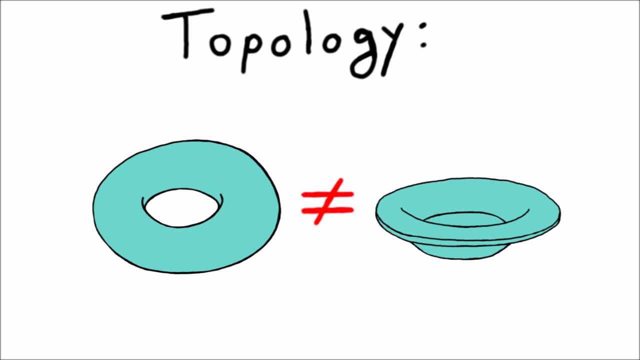 tell the difference between a donut and a pie plate, For example. we don't care that one is made of metal and the other is made of delicious doughy goodness, But we care very much that one has a hole and the other doesn't. 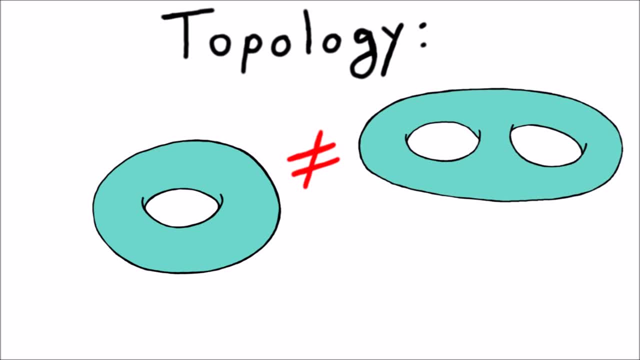 We can also distinguish between a donut and some kind of ultra-delicious donut with two holes or three. We can also distinguish between different kinds of holes because holes behave differently in different dimensions. If I snip a hole in a piece of thread, that's different from poking a hole in. 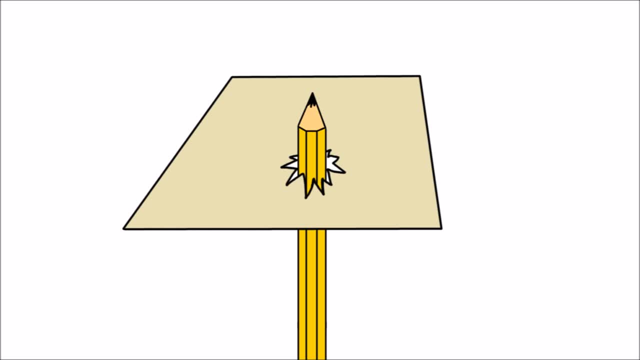 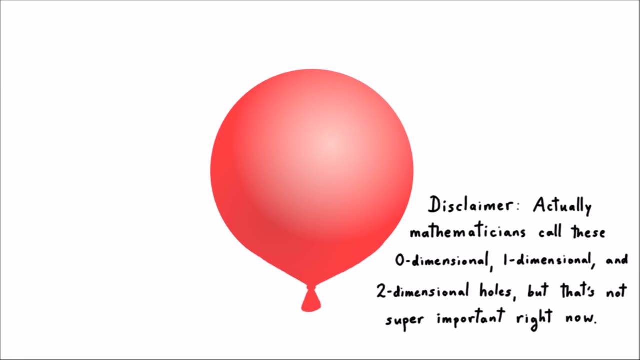 a piece of paper, for example, and those holes are both different from the kind of hole that forms inside a balloon when you blow it up. we can think of these as one-dimensional, two-dimensional and three-dimensional holes, And there are ways of studying holes in other dimensions as well, By choosing to ignore certain 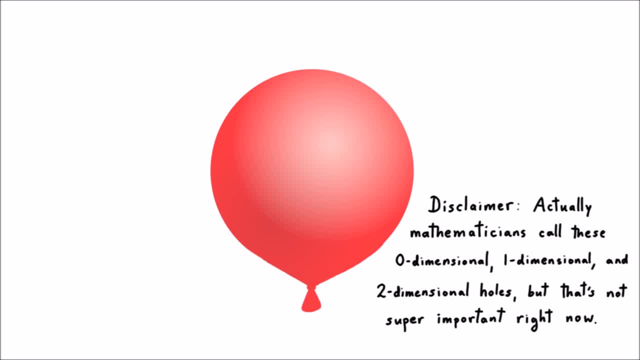 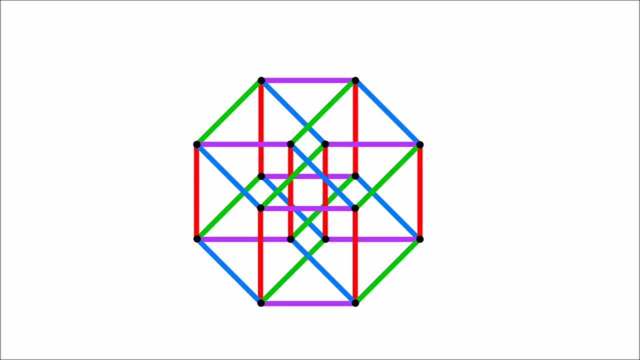 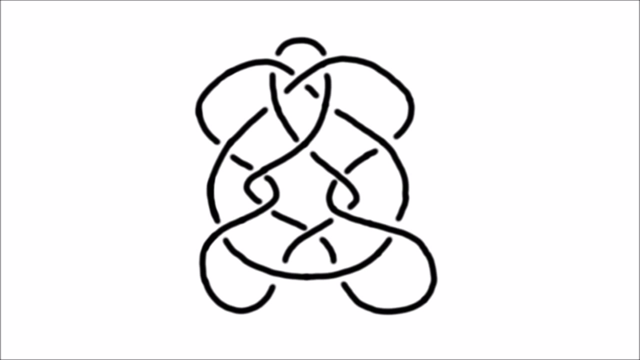 details about shapes, we can focus our attention on their more fundamental properties. This is especially important when we study crazy shapes, Shapes like high-dimensional objects or curved models of our own universe, or complicated knots, or, say, knotted surfaces in a curved four-dimensional. 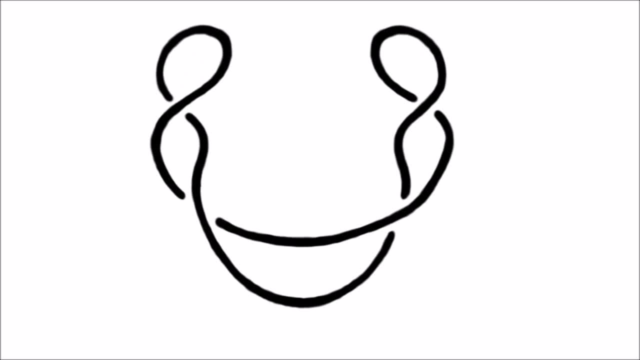 space. If you're studying the Sistine Chapel, you don't want to spend your time carefully measuring every brick, And when you're trying to wrap your mind around a very crazy shape, you want to be able to focus on the features that matter to you. At the same time. studying topology doesn't mean 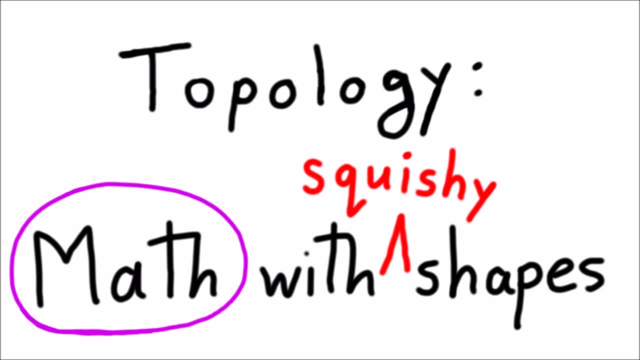 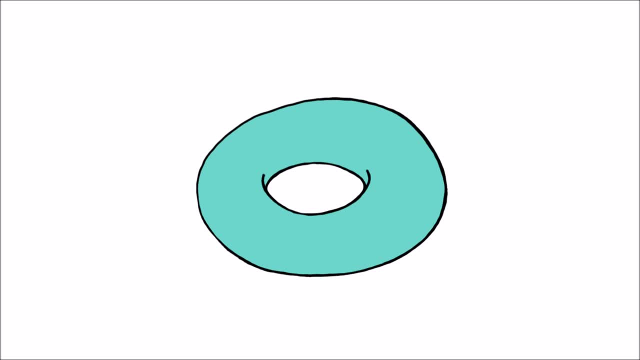 throwing out rigor. We choose to ignore certain information, but we need to be very careful in how we do this to ensure that we're being consistent. For example, if I make a donut out of Silly Putty, I could crush the hole closed and then flatten the shape into a plate. But a donut and a plate.